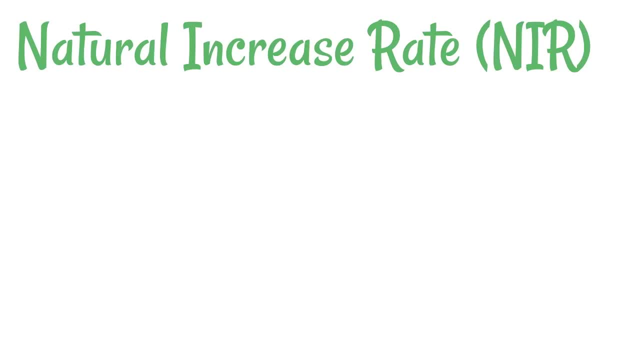 rate. Now this is a way we can use crude birth rate and crude death rate to give us some useful numbers as to how things are changing. So this is the rate of human growth expressed as a percentage change per year. Notice, it's a percentage change. So let's go back to our data. 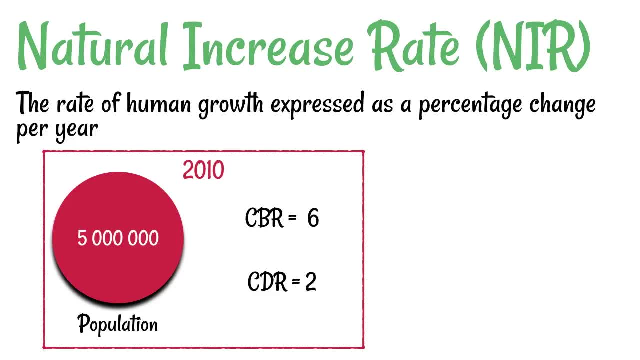 for this nation. We've already calculated our crude birth rate and crude death rate, which we've got here Now. to get the natural increase rate, we've got to do the crude birth rate minus the crude death rate. We take that number and we divide it by 10 because we don't want to be using 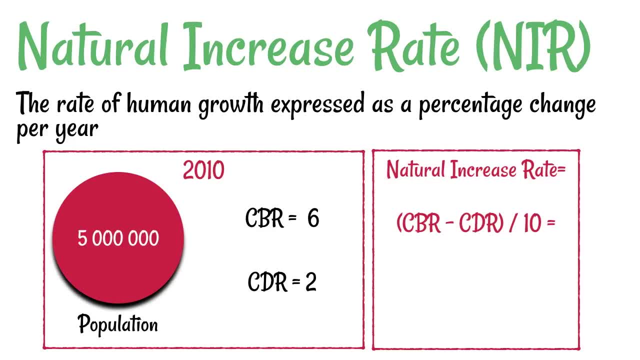 values per thousand, which is what crude birth rate and crude death rate are, but we want to convert it into a percentage, So 1,000 divided by 10.. So we're working with out of 100, which is a percentage, 6 minus 2 divided by 10. for this: 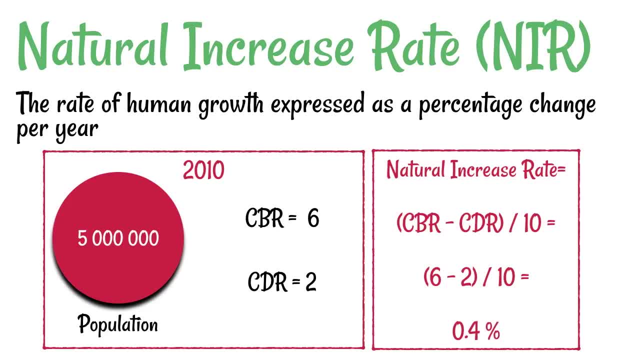 population gives us 0.4 percent. Now what that means to us in the real world is that this population will increase in size by 0.4 percent per year, assuming that these conditions remain the same, Assuming that the crude birth rate and crude death rate remain constant. Another: 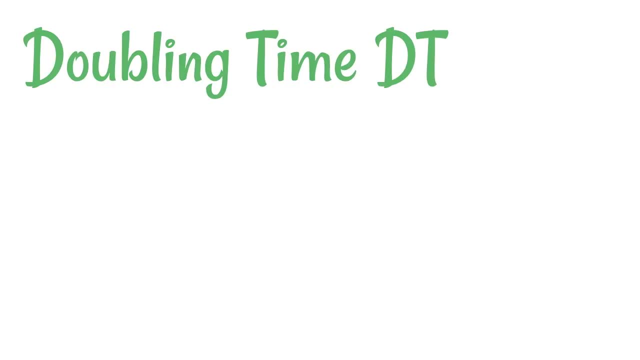 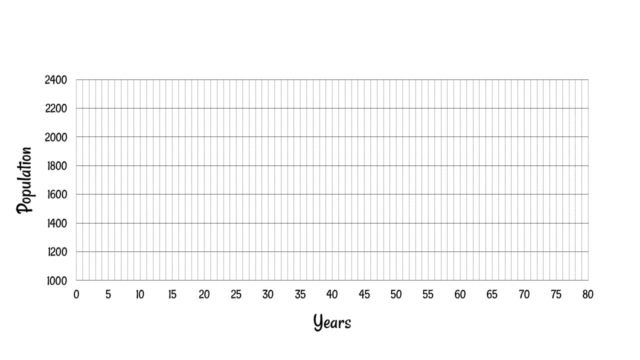 important idea is something called doubling time, and this is just simply the time it takes in years for a population to double in size. Let's look at a really simple set of data and let's say we've got a 1 percent increase per year. So that's a natural increase rate of 1. 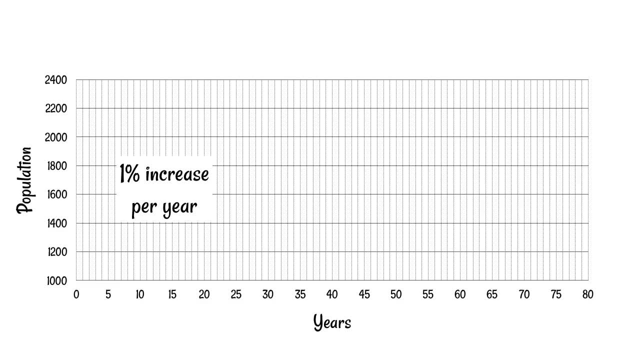 percent. We start off with a population of 1,000 and as they increase by 1 percent per year, this is what their population growth will look like. If we want to find the doubling time, all we've got to do is go up to a value of 2,000, because that's we started with 1,000, so we're going to 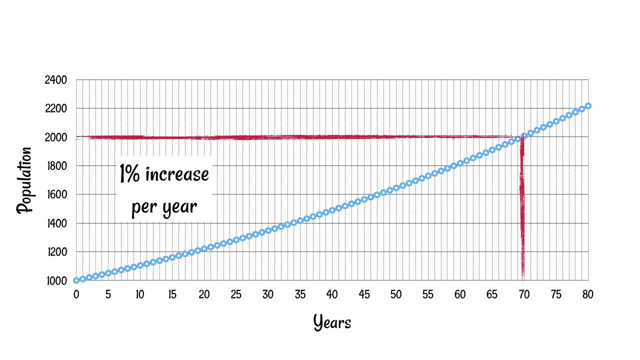 double that, which is 2,000.. Read that off the graph here and notice that the time it takes to do that is 70 years. Now this is a really, really important number. It doesn't matter what size of population we begin with. If there is a 1 percent increase per year, the doubling time will always be. 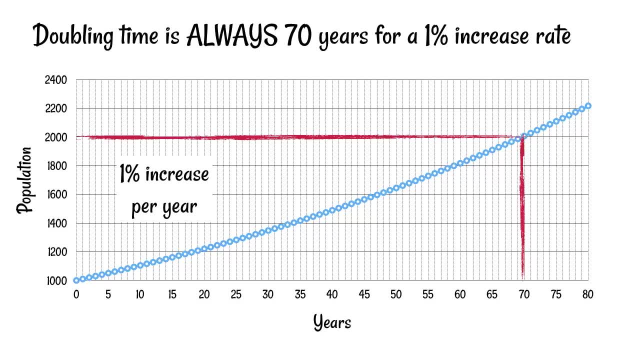 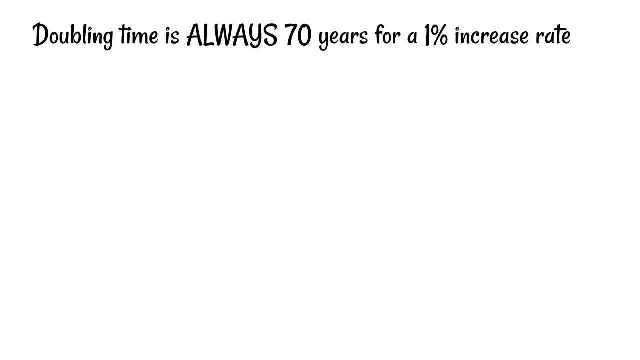 70 years for that population. Now, because that value is constant. that makes it really, really easy to calculate doubling. Let's use our original population as an example here. Doubling time is equal to 70 divided by the natural increase rate. That's where that that number 70 comes in really handy. So for our 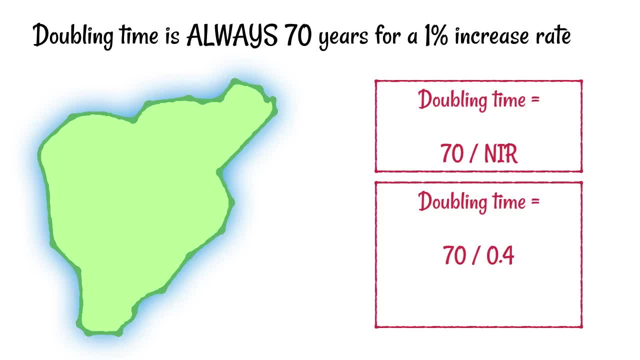 population. we've got 70 divided by 0.4.. That's the natural increase rate we calculated for this population. 70 divided by 0.4 gives us a doubling time of 175 years. What that means is it'll take 175 years for the population to double. So that's a really, really important number. So that's a 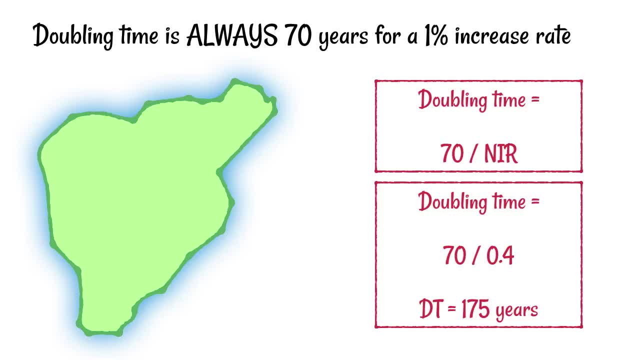 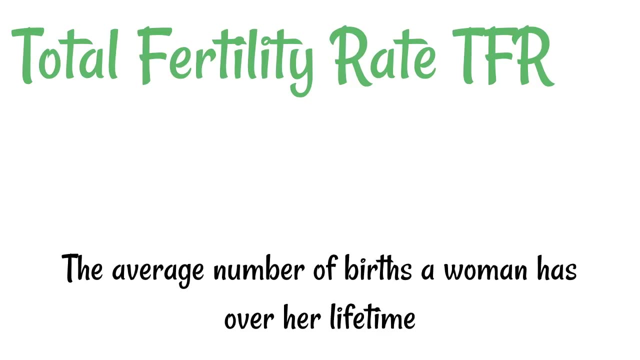 particular population to double in size, assuming that those values of crude birth rate and crude death rate remain the same. Another important value when considering population dynamics is the total fertility rate, and that is the average number of births a woman has over her lifetime. Now let's imagine we've got a total fertility rate of two, and what that means is that the 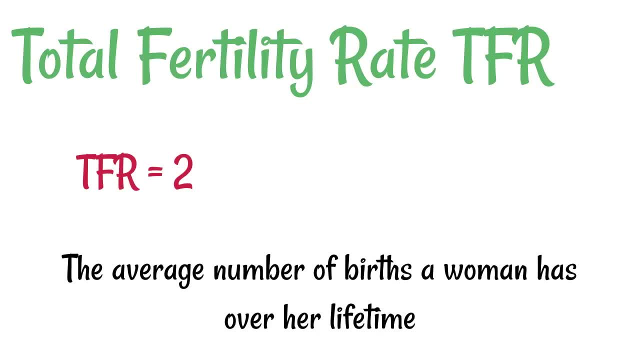 average woman in that population will give birth to two children in her lifetime, So this couple have two children. That means that this woman has replaced herself in the population, and it also means that she has replaced her partner in the population, and so our population size would remain. 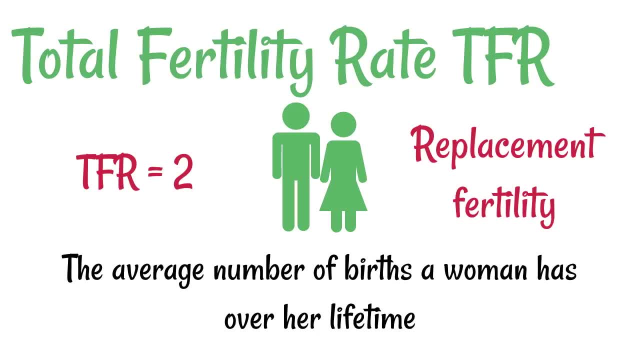 constant. So this number two can be considered as the replacement fertility. However, this is not strictly accurate. In actual fact, the numbers are a little bit different. In MEDCs the replacement fertility value is around about 2.03.. It's quite close to 2.03.. So that's a little bit different. 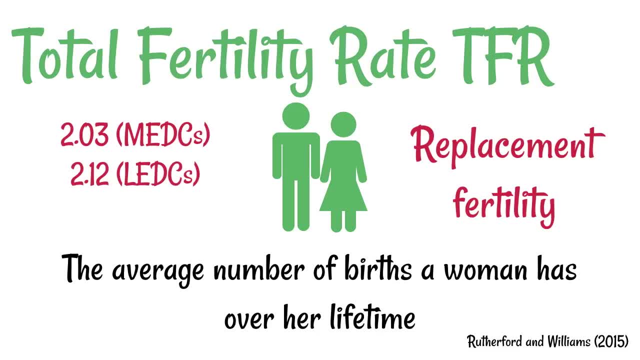 In MEDCs it's a little bit higher, 2.12.. The reason for this is that not all children are going to grow up to be adults. We have to take infant mortality rates into consideration, The reason that values are different for less economically developed countries and more economically 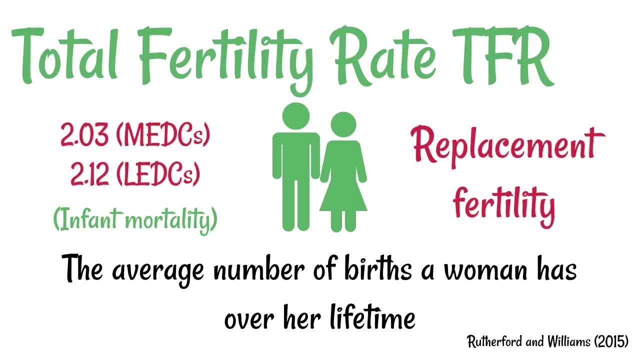 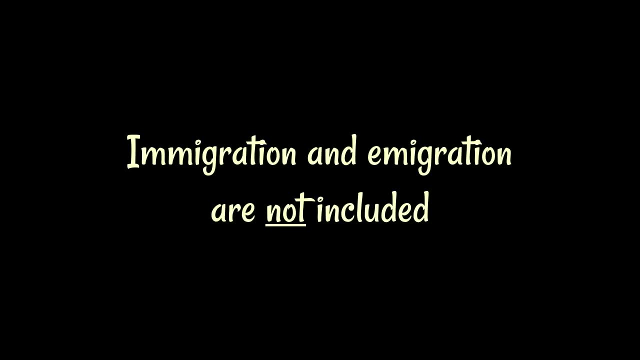 developed countries is that the standard of health care is lower in less economically developed countries and therefore we would expect the infant mortality rate to be higher. It's really important to note that, amongst all of the countries that we're talking about, all of these calculations, immigration and emigration have not been included. We've assumed